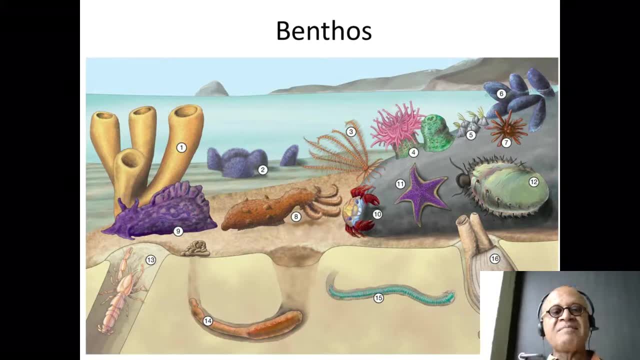 are very still okay. So here are some examples like these. attached to the bottom. They look like tube worms. You can see some barnacles here, sea urchin, clams and so on. So these are the sea urchins. You can see some starfish here, crab, here, some worms that have buried. 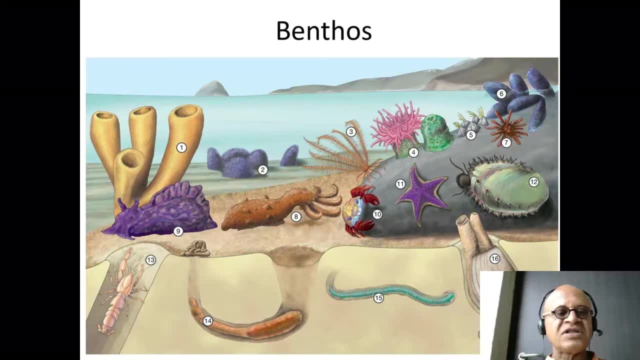 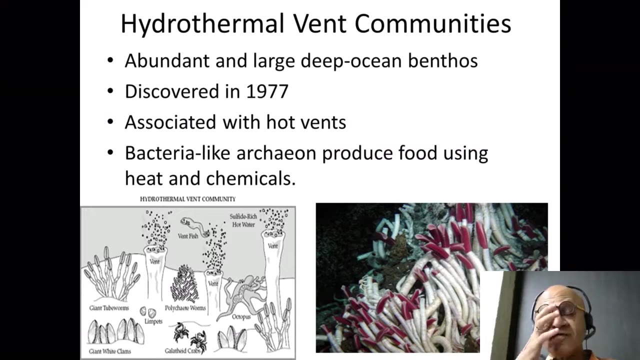 themselves into the sand. This is called some kind of a crab that actually stays buried inside, as opposed to this crab which is on top. okay, So this is kind of shallow coastal water, but you can also find life that goes very deep in the ocean. I'll show an example. 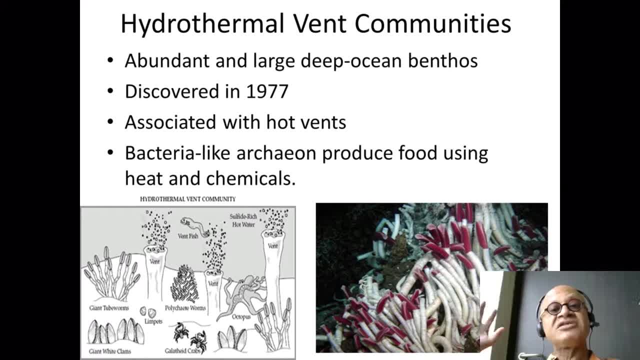 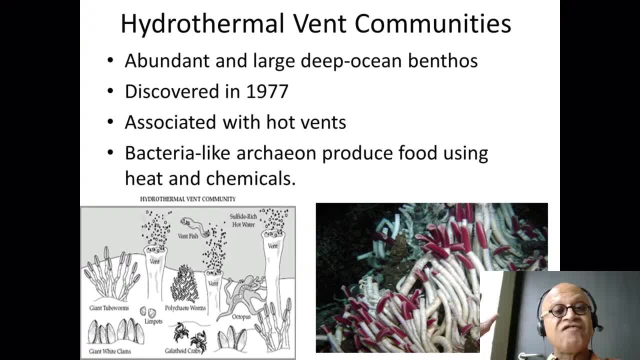 flesh that can be eaten dies and falls to the bottom of the ocean. Who eats it? You'll see that there are many snaky-looking things that keep chewing on this whale meat and eventually microbes come in and eat whatever remains and then some other microbes can chew into. 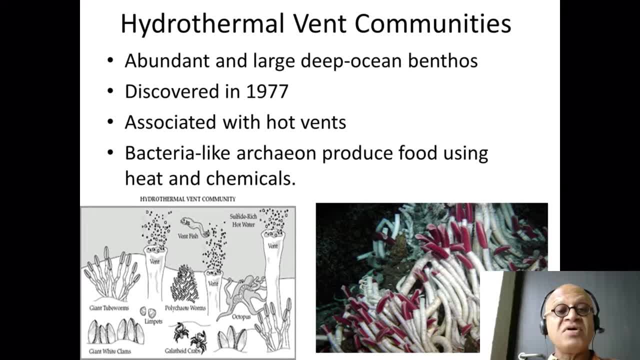 the bone and the whole thing gets destroyed over time. but that is a lot of food that comes down to the bottom of the ocean. The other interesting habitat in the Bantos is the hydrothermal vent that I already mentioned. You can see some tube worms here at the hydrothermal vents. 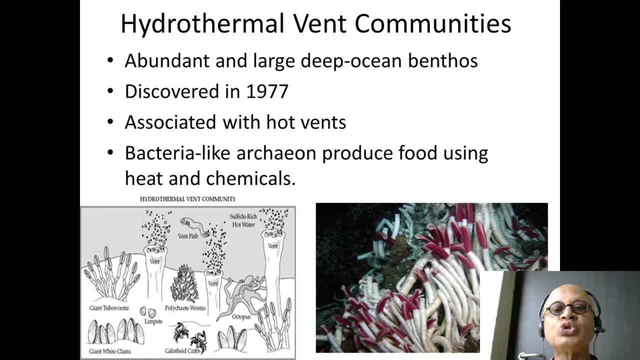 They were discovered. the deep ocean hydrothermal vents were discovered in 1977. It turns out that there are many in Galapagos, in Baja California. There are hydrothermal vents in many places, which is related, again, to tectonic activities. 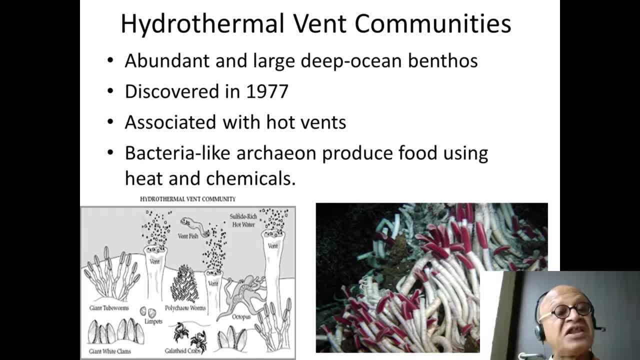 That's where the toxic stuff can come from, within the bottom of the ocean, into the water column right, So they're associated with hot vents. so energy has to come from below And there are bacteria like archaeons. They produce food by using heat and chemicals. 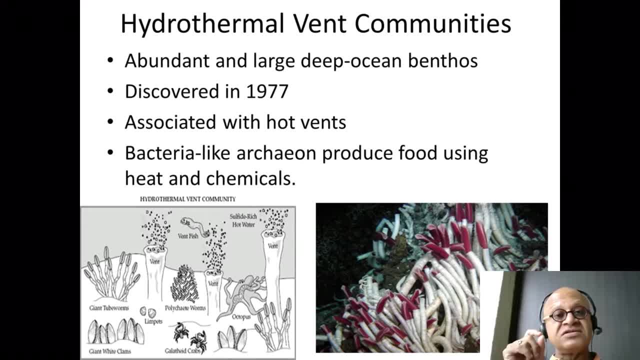 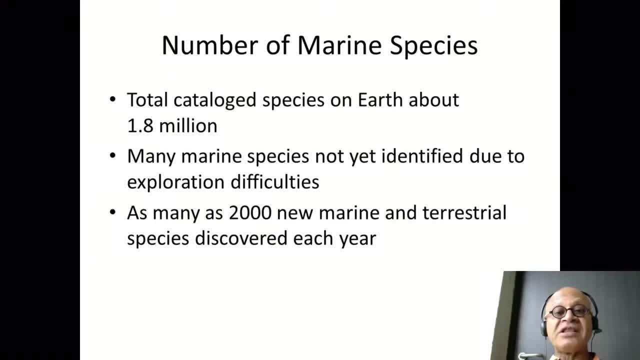 So remember, there is no light here, so there is no photosynthesis, but there is chemosynthesis. So we will look at the chemosynthesis equation later on in the next chapter. So let's take a look at the number of marine species. 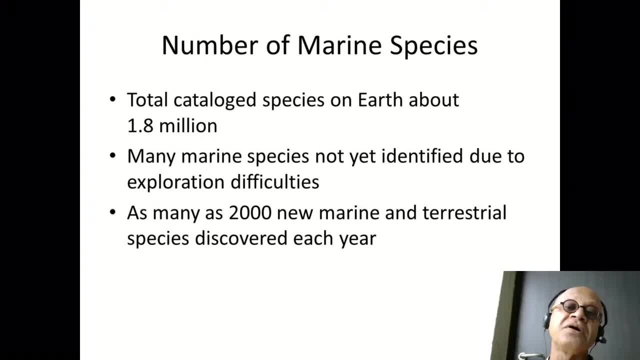 Here is something interesting: You can bring back your concepts of how the ocean changes And Something we repeated several times: that the ocean has a very high heat capacity, so its temperature changes slowly, right, And we said its salinity doesn't change a lot except in hypersaline lagoons and so on, where seasonal cycle can be very large because shallow waters can rain during one season and can evaporate during another season, and so on. 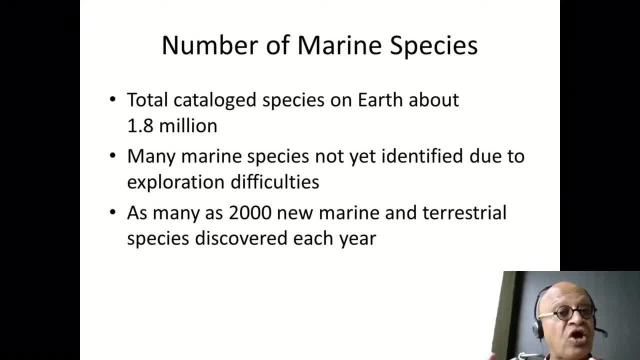 So the marine environment doesn't change. It doesn't change a lot except at the bottom. Okay, How does that relate to the number of marine species, Compared to the very rapid and very quick changes on land because of the low heat capacity? 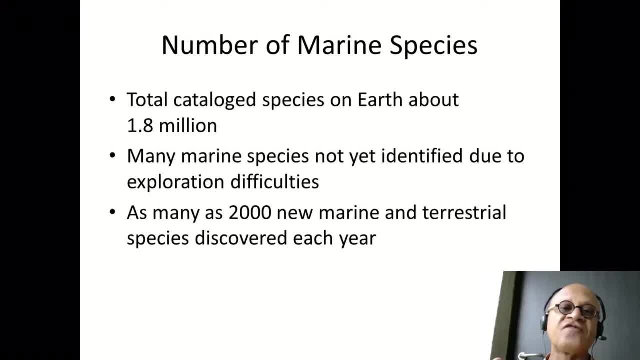 out of the total catalogued species of about 1.8 million. this number will keep increasing because we discover new species every year And so many more species are not yet identified. And so many more species are not yet identified Because we don't have enough species. 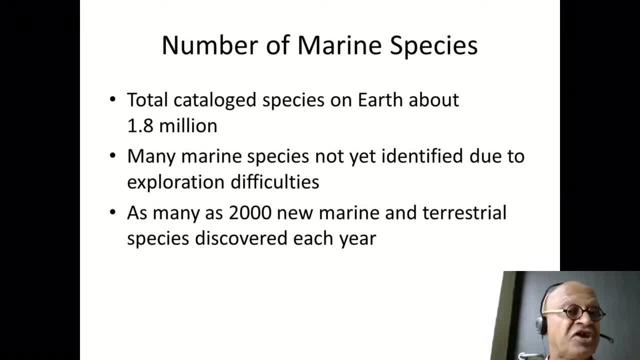 And so many more species are not yet identified. We haven't explored all of the heavy rainforests or the deep deep ocean. So almost 2,000 new marine and terrestrial species are discovered each year. So this number will keep growing. 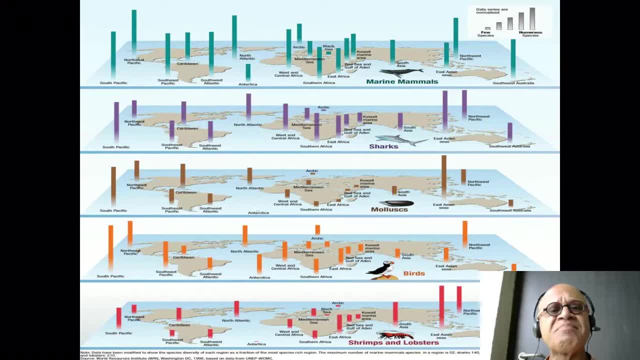 There was something called a consensus of marine life, C-O-M-L, that was done in the last previous decade with a budget of $650 million And it And it discovered all these species. So you can see that, the numerous species, you can see the different heights of these bars. 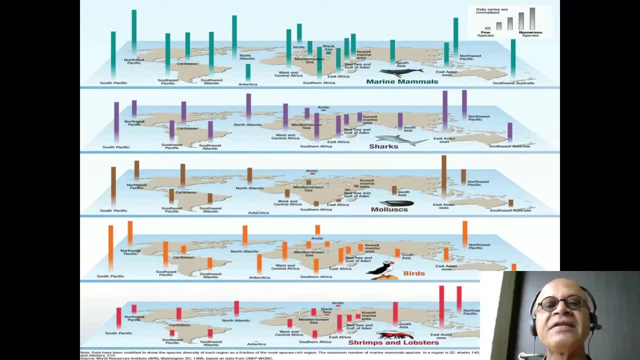 Okay. So the challenge is always to understand what determines the biodiversity or the number of species in a different place. So this is just marine mammals. These are the different types of sharks. These are mollusks, Birds- Yes, Birds- These are the birds that predominantly live on marine resources. are called seabirds. 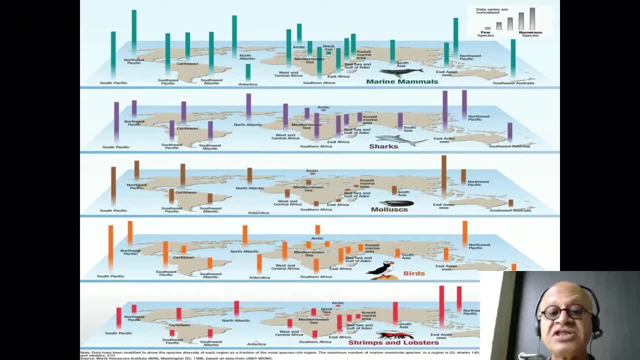 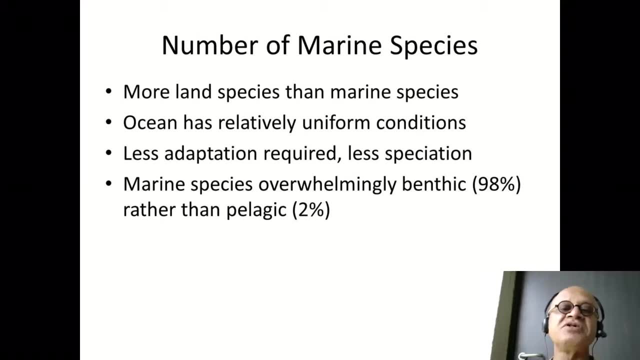 Okay, And shrimp and lobsters. So you can see the global variations in the number of species. Since the land is highly variable, you expect that most of the species will be found on land, So the number of marine species will be much smaller because of this relatively uniform temperature. 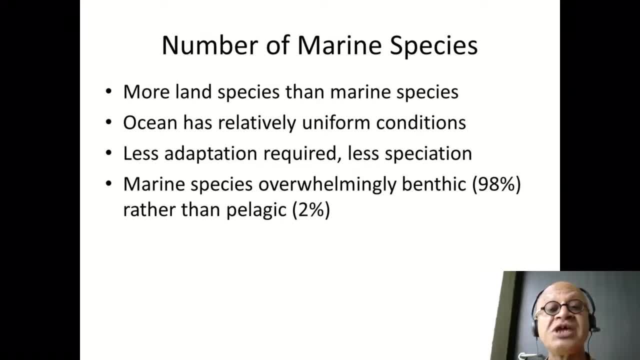 And temperatures and salinities that change do not change so fast. Right, So life evolves to fit into environmental niches. Something happens like a meteorite crash or an earthquake or whatever else that changes conditions for a longish period Or an invasive species that you move from one location to another. 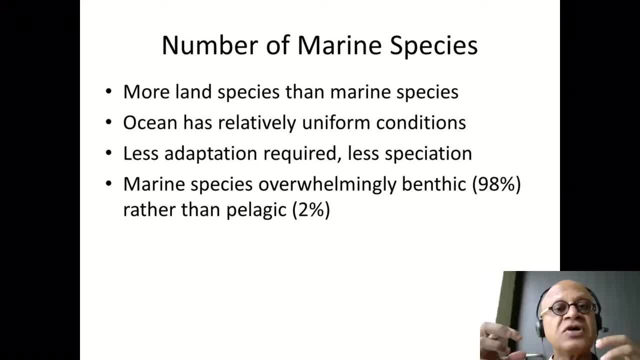 Then if new environmental niches, new temperature, new salinity et cetera evolve, new level of light et cetera, then new species evolve. So, as Darwin said, it's not the strongest species, it's not the smartest species, but the: it's the most adaptive species that survives. 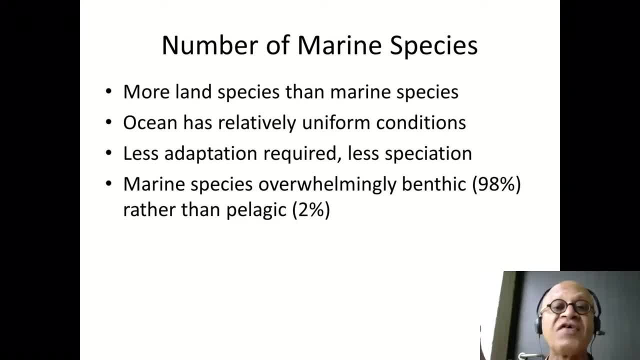 Right. So ocean this way ends up with very few environmental niches and much fewer species. So less adaptation is required and less speciation evolution of new species, And that's what we're going to talk about in a little bit. So let's talk about marine species. 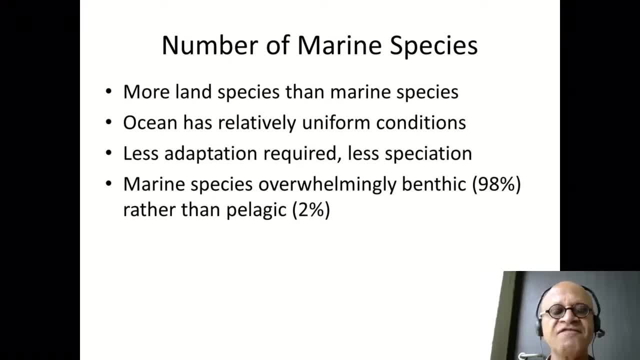 So marine species are overwhelmingly benthic. So if you take all the marine species, then 98% of them are on the bottom because, as you can imagine, the water column cannot change very fast, but the bottom still changes very fast. 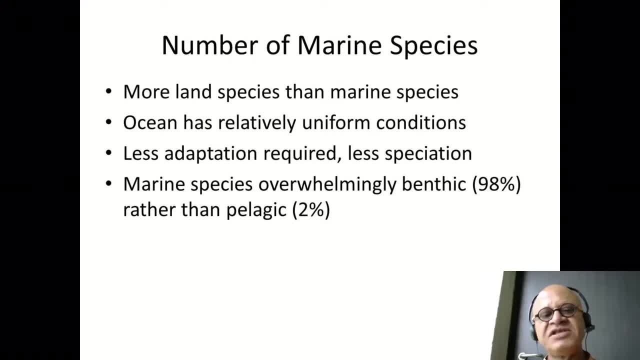 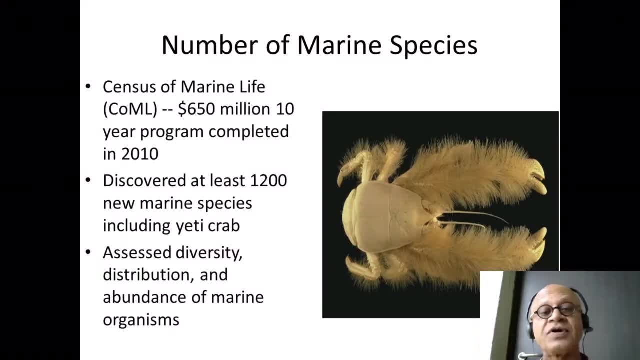 So 98% of all marine species are at the bottom And only about 2% are in the water column. So 98% of all marine species are at the bottom and only about 2% are in the water column. Okay,